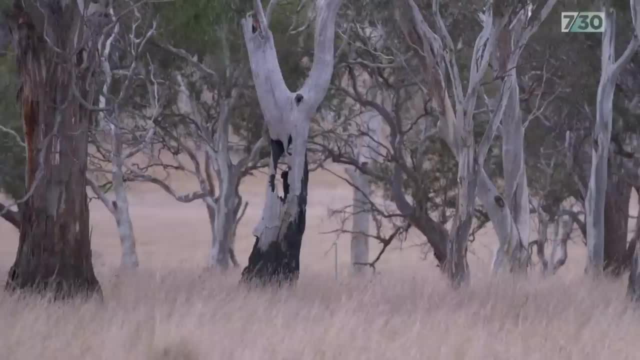 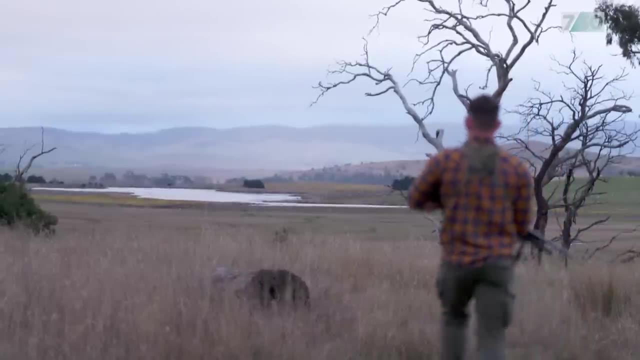 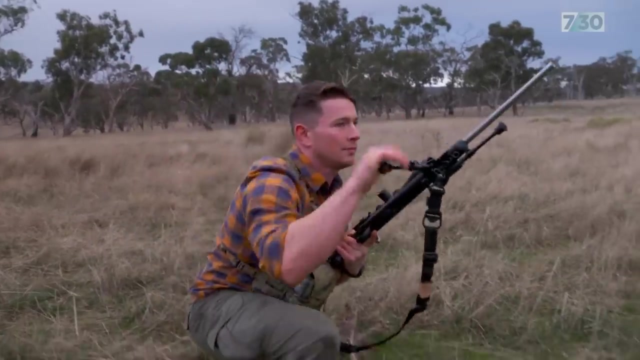 None of my guys are out at the moment, so you've got the run to yourself. While other states and territories recognise deer as a feral pest, in Victoria and Tasmania established wild deer are managed as a game resource and are partly protected. 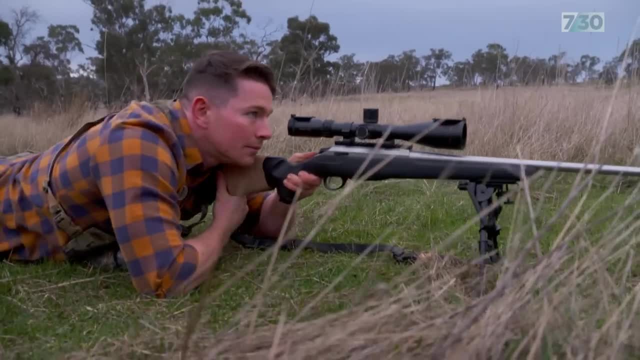 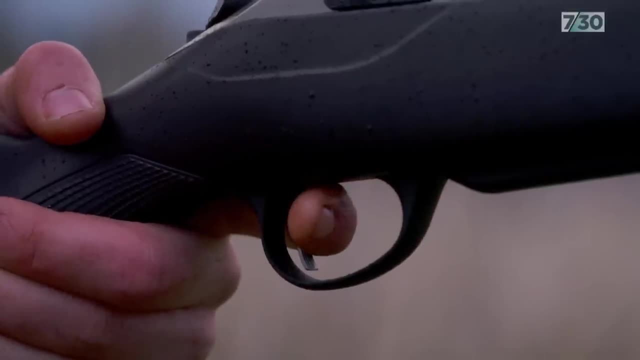 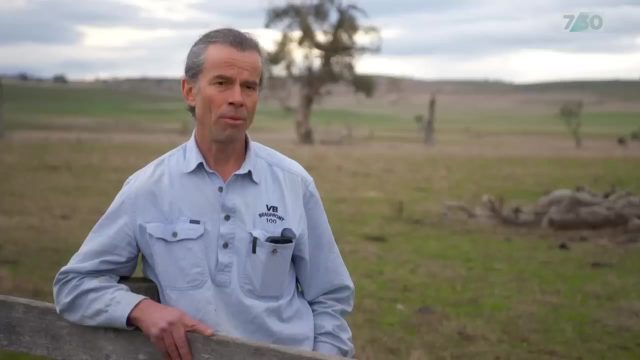 Victoria has made it easier for landowners to shoot problem deer, But in Tasmania landholders have to apply for crop protection permits and hunters need a game licence to shoot during a limited season When we're unable to shoot them because our permits have run out. 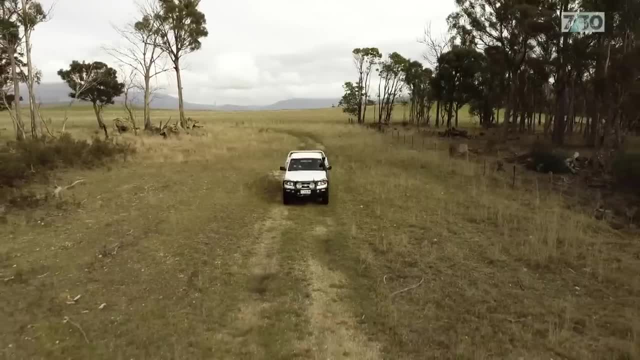 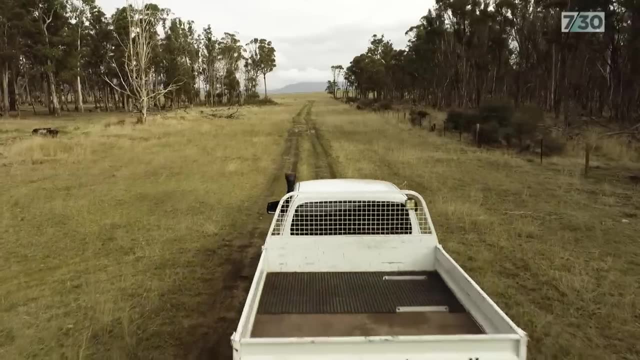 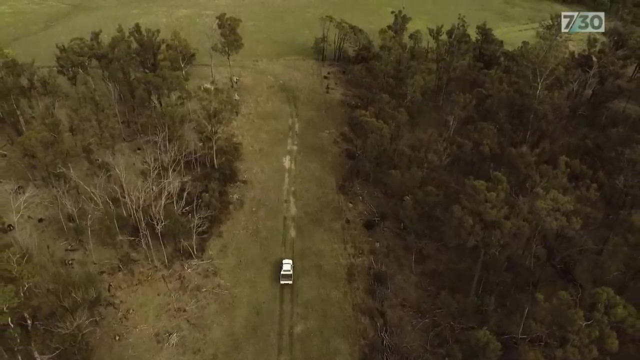 then they come back again. Scott Freeman is a third-generation hunter. He doesn't want deer declared a pest, but he believes game hunters should be playing a role in getting deer out of Tasmanian national parks, as they do in other states. 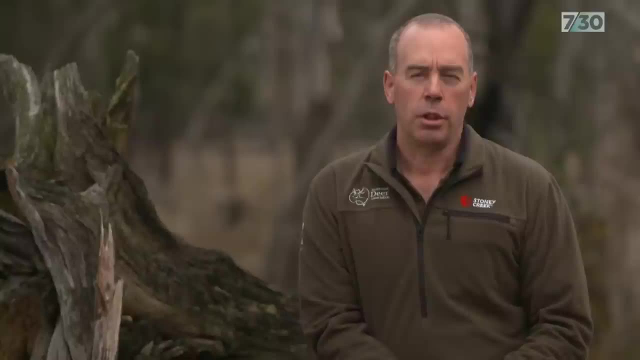 A lot of that's done at night with night vision gear. We'll go in and control those areas and all the meat is recovered through those programs and taken home and utilised by the program participants. It's not just rural areas with deer issues. 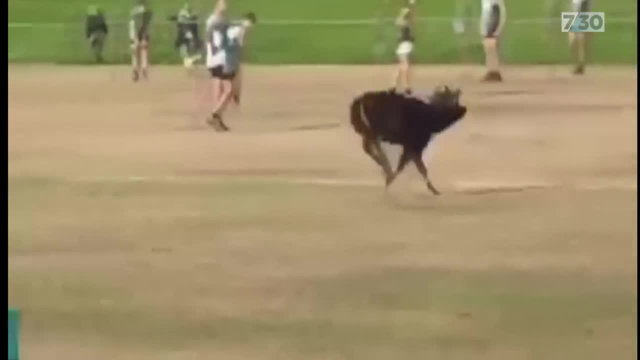 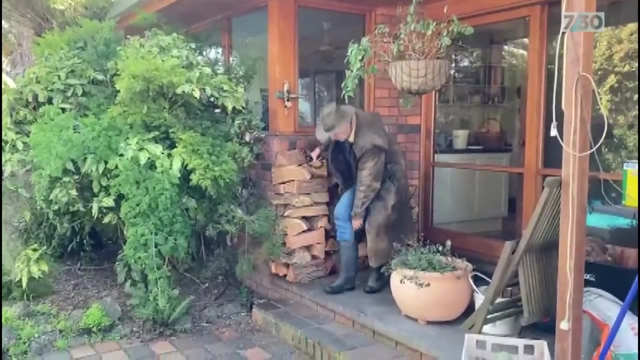 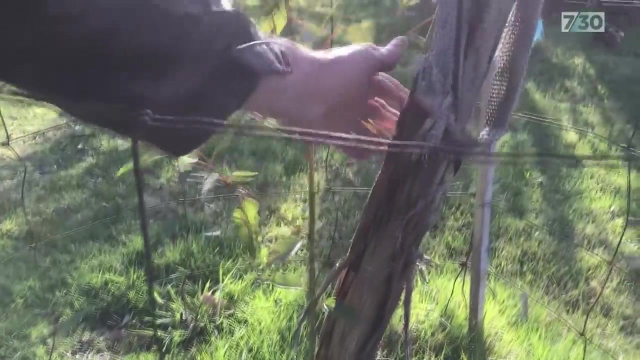 In recent months they've been spotted in inner Melbourne and at a suburban football game. Johannes Wenzel lives in the Dandenongs, effectively outer Melbourne suburbia. About five years ago he noticed his rose bushes and fruit trees were being pruned. It took us quite a while to wake up that this was actually deer damage, And then it really went rapidly up and it has become a huge problem in our environment. Local residents have been reporting vegetation damage and deer on roads. Deer have also eroded embankments. 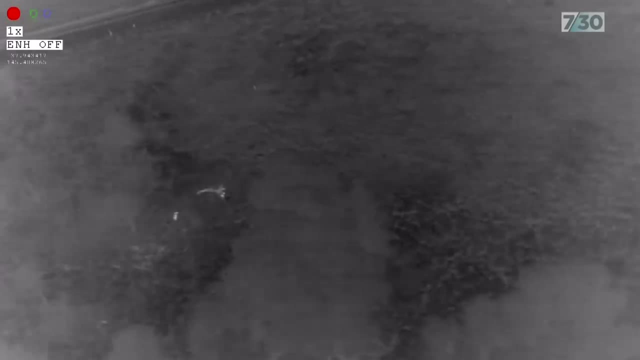 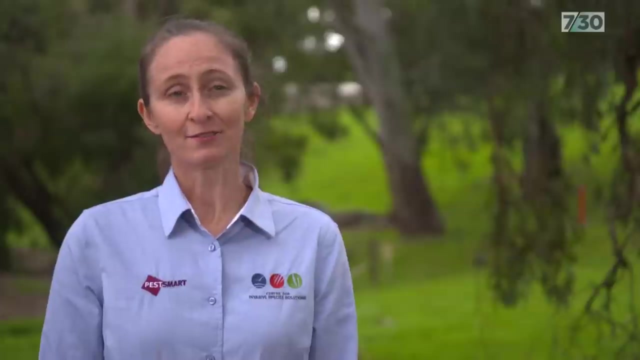 and browsed where lyrebirds normally nest. Results from an aerial survey estimated more than 1,600 deer in an area of just 110 square kilometres. It's a really big problem to manage deer in urban and peri-urban areas. At the moment, the main tools for managing deer 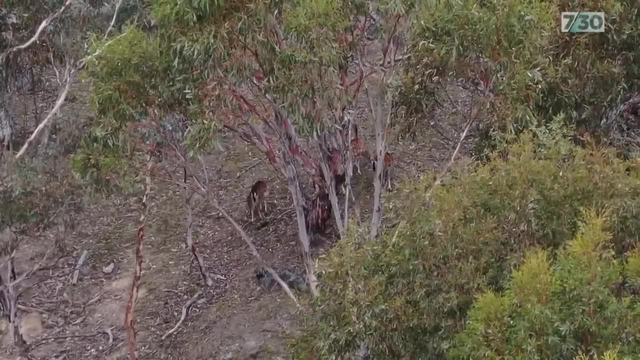 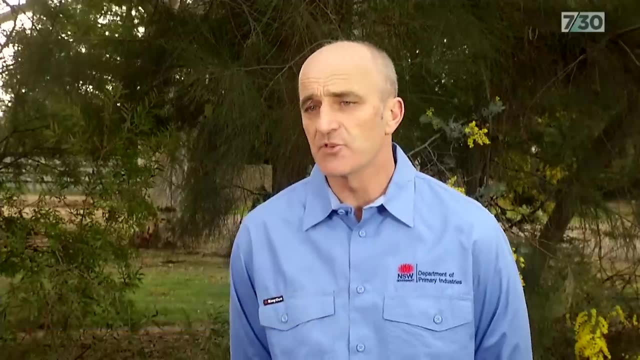 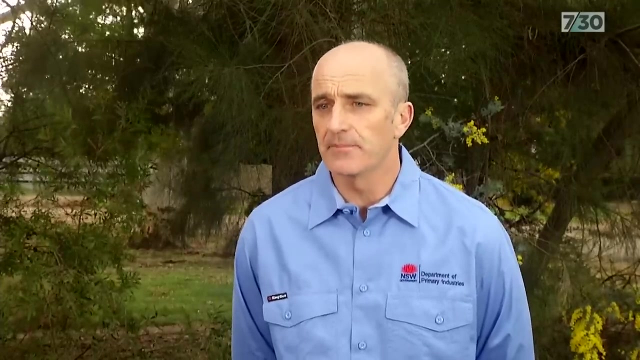 are really to shoot them or to trap them or fence them. Ground-based shooting at night using professional contractors is effective, as can be some trapping and fencing, But in larger, more remote areas, for example national parks and large pastoral properties.